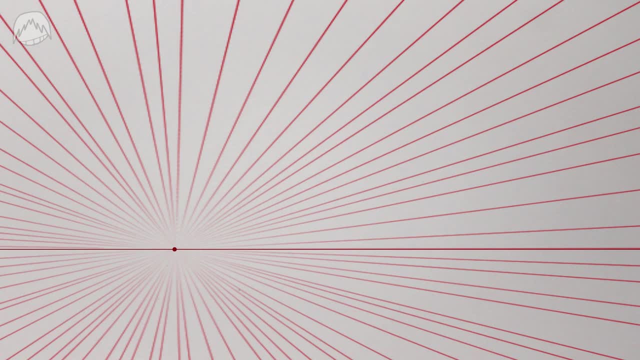 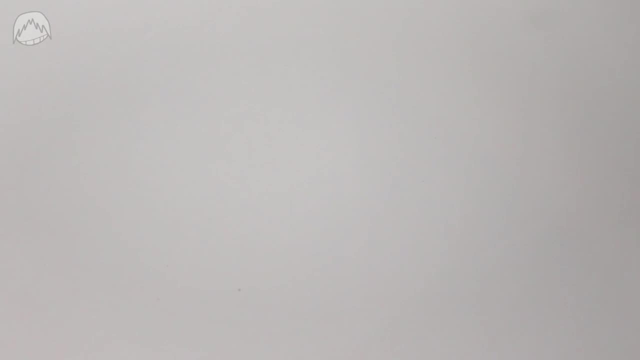 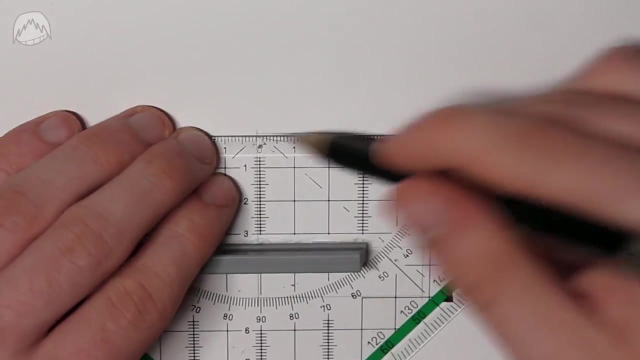 attracts all lines that go in this direction. That's a new rule we're gonna establish in this drawing here. Now let's start with something easy. So we're not starting with a building or something, but a very simple, easy rectangle. And now we're transforming this 2D rectangle we just drew into 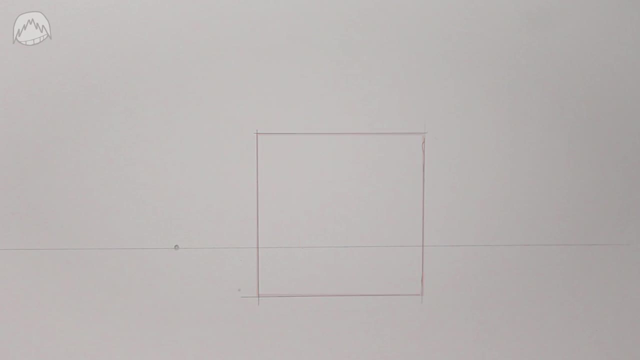 a 3D cube. To transform this 2D shape into a 3D one, we need to add another plane to this object, And this new plane points towards the vanishing point, And now you get to decide where to cut it off. 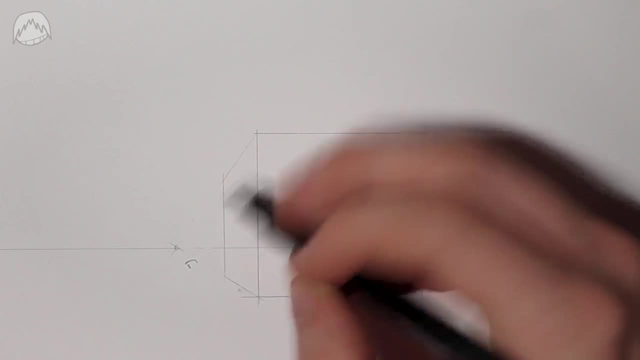 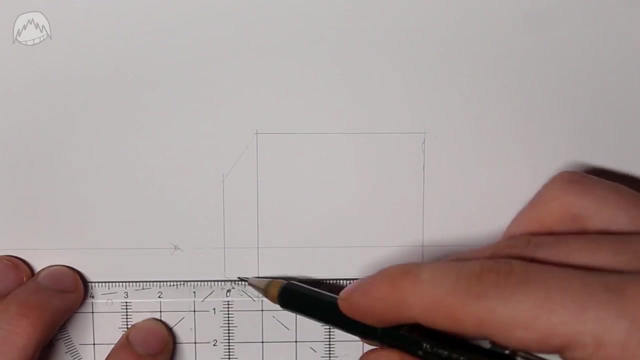 Also, just a tip for you guys always draw the wireframe, so basically the skeleton of this drawing. Just draw it the same way I do. With a bit of practice you get a hang out of it. Believe me, I know all of you think. 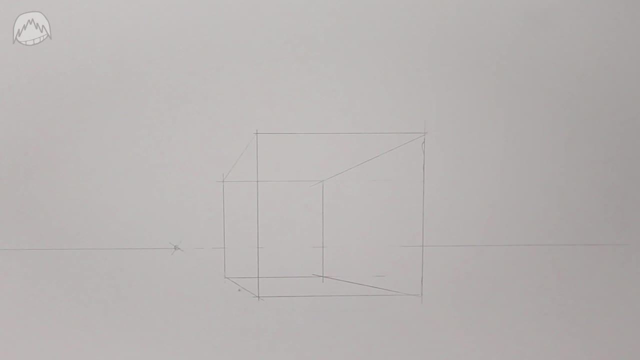 that drawing this wireframe is completely unnecessary, but you'll be thankful you did it later on. For example, when you want to draw another object behind your drawing, you can use those lines as guidelines, And yes, this also works with objects that lie on top. 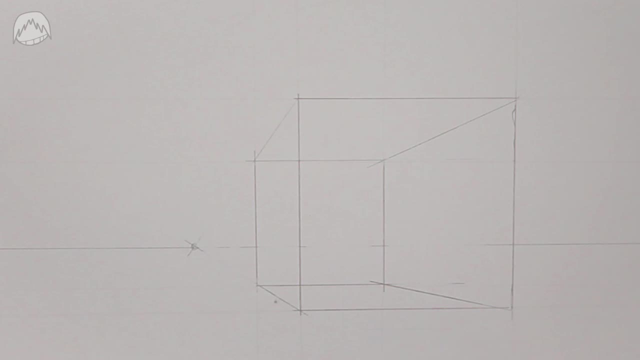 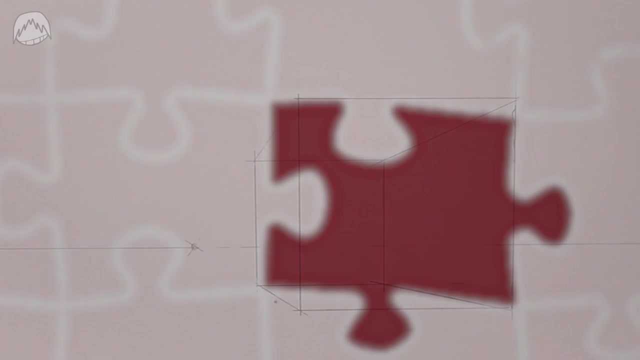 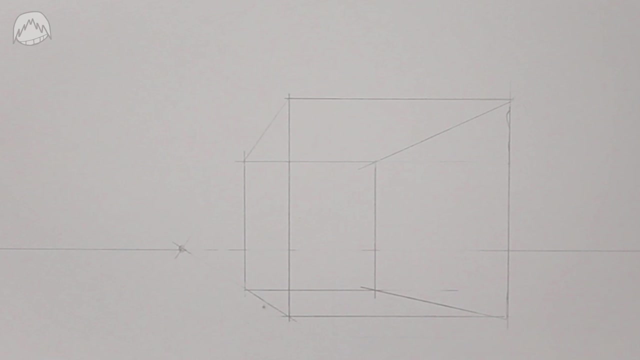 or besides your objects. Just envision it as a puzzle. The object you just drew is piece number one And based on this object, you can kind of figure out where the other pieces go. By the way, when you're only using one vanishing point, you need to make sure that the other lines 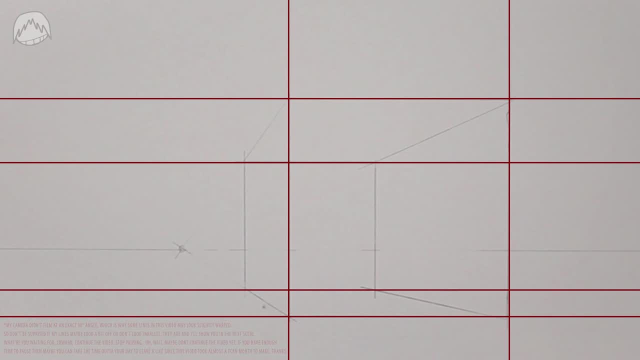 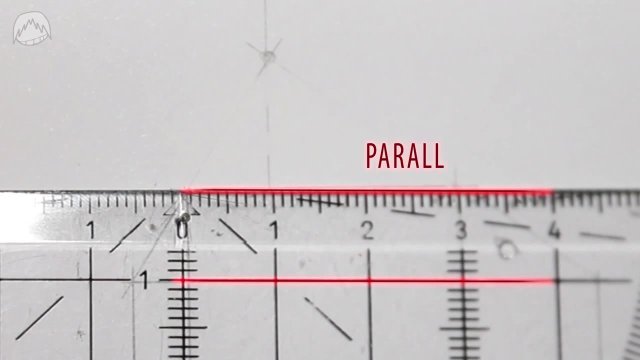 are parallel to each other. Like I just showed you, you're using those lines as guidelines later on. So if those lines are off, your whole drawing will be completely wrong. You can always use a triangle ruler for your perspective drawings, So just make sure you. 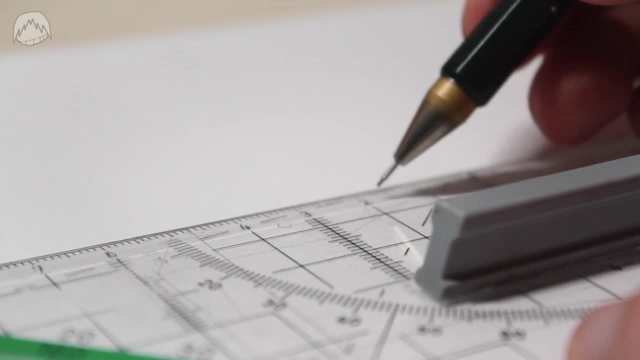 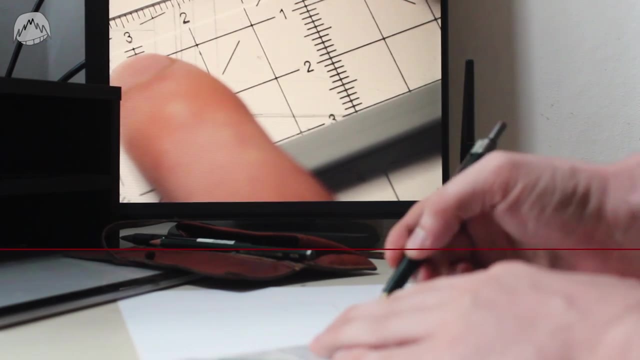 understood everything up until now. You can also go ahead and try to draw along, so that you are getting some practice out of this as well. Oh, and maybe you've been wondering what's the deal with the horizontal line? Up until now, this thing was pretty useless, wasn't it? So what's it? even 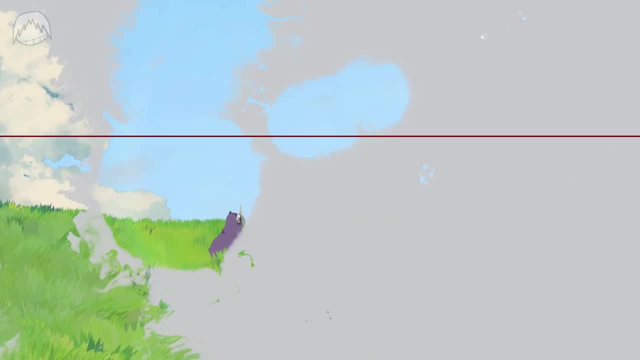 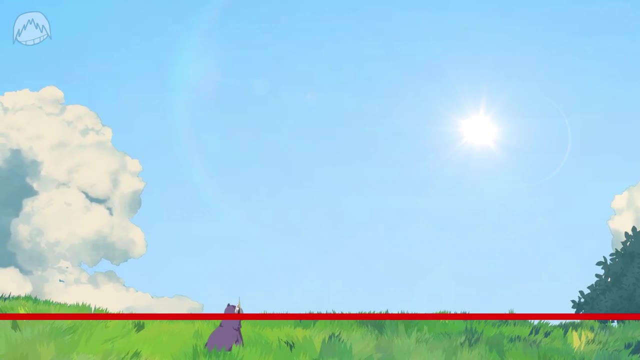 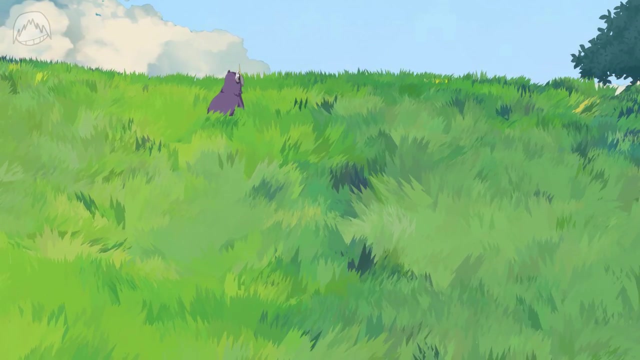 for Well, your horizontal line determines the height of your artwork. Just imagine it like this: if you're looking up Upwards, in real life, the horizon is further down, And if you're looking downwards, the horizon is at the top part of your view, And the same goes for your art. If the horizon line 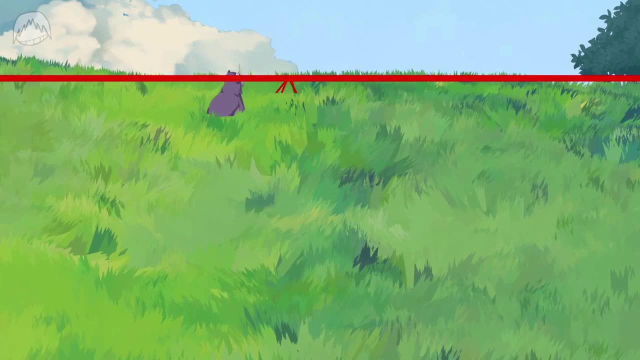 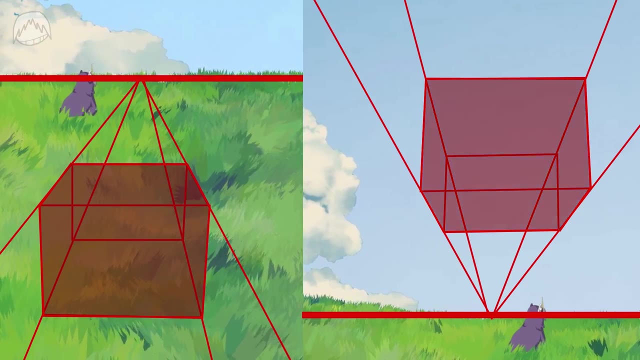 with the vanishing point are on the upper side, you are looking down on your object, And vice versa. if the line is at the bottom, you're looking up to your drawing And yeah, of course, if it's in the middle, you're looking directly at your object. 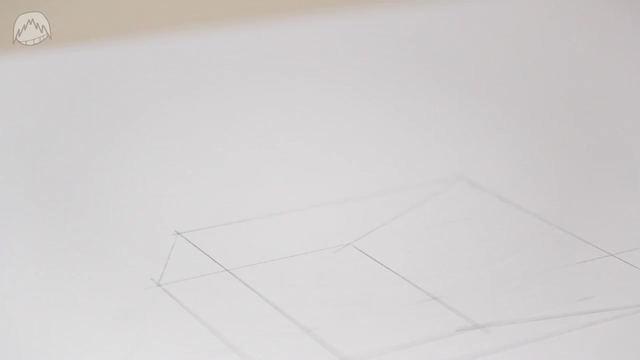 but you could have figured that out yourself. Now, the first thing towards understanding vanishing points was the most important one. Now, you can draw anything with a one point perspective, Like, for example, you can make this cube into a house by adding a street Using a vanishing point. 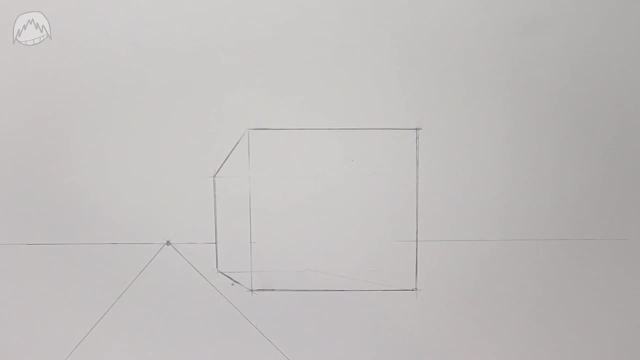 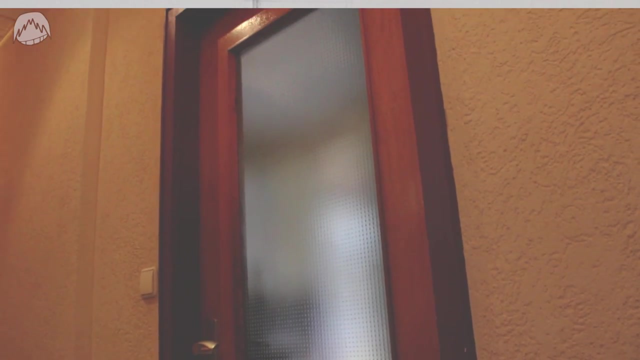 you should be able to draw a simple street without a problem, And you could also add a roof, And the same also goes for a door. Before we go to level two, there's something I have to do To show you first, and that's the details. If you take a look at a door in real life, 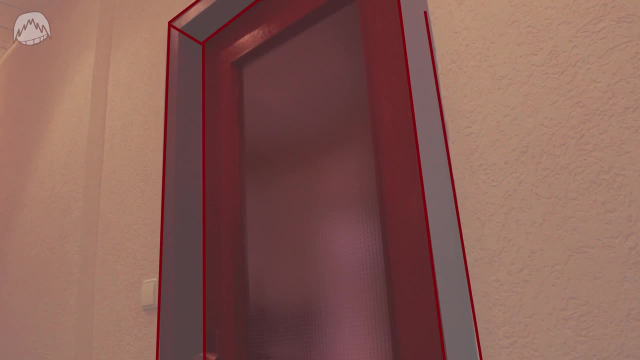 it's not completely flat, but it has depth to it Because it's 3D. So try to form a habit of drawing things more 3D in your art as well. Let's try it out by drawing this door in the. 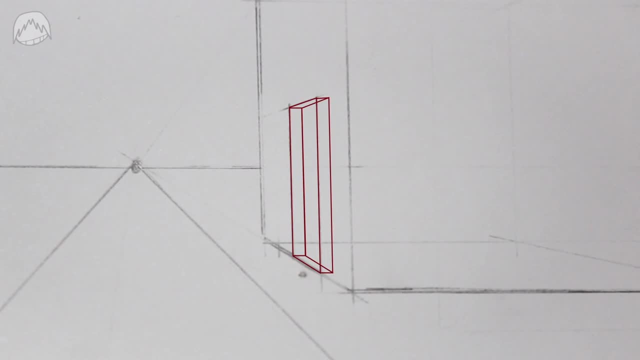 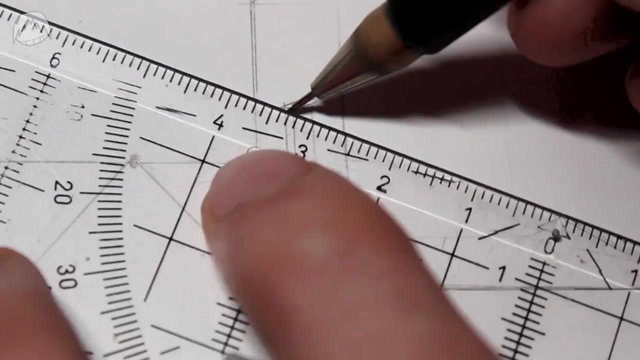 third dimension. Try imagining a box here, like we did with the previous example. Start off by, for example, drawing the horizontal lines, After that add the vertical lines And lastly we add the lines that go towards our vanishing points. 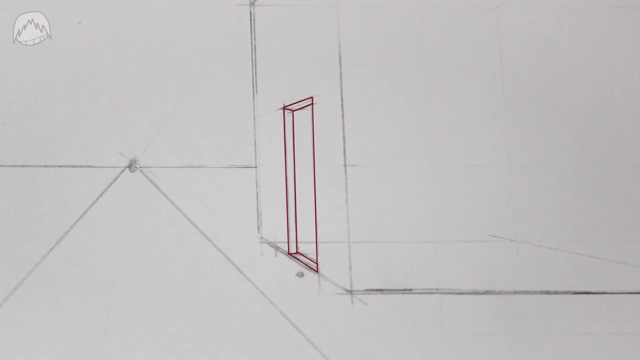 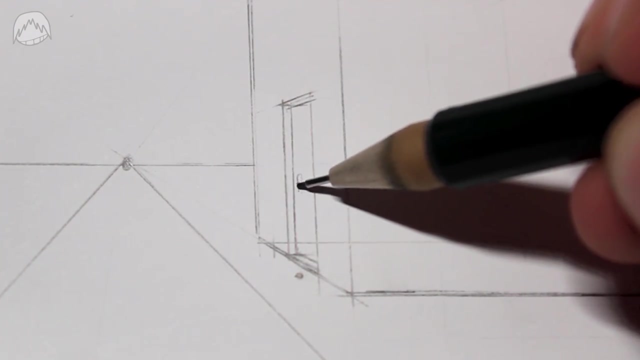 Don't worry, there's no particular order to it And the rest you don't need to draw If you don't want to, since you can't see it anyway. I'm sorry if you already knew all of this, but some people are still beginners and might be. 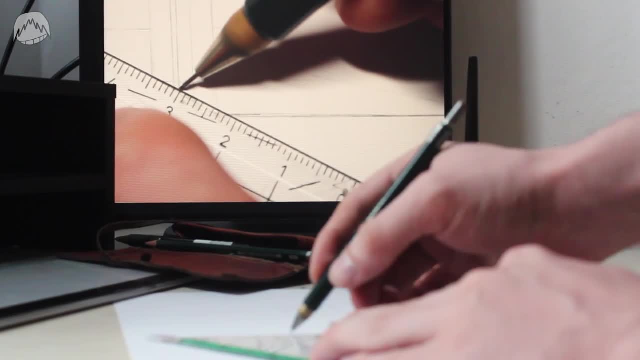 really grateful for that knowledge, so I wanted to include it here. If that's all new to you, then it can be a bit much. So try practicing what I just showed you and you'll be able to draw a lot of things. If you want to see more of this, then click here, And if you want to see more, 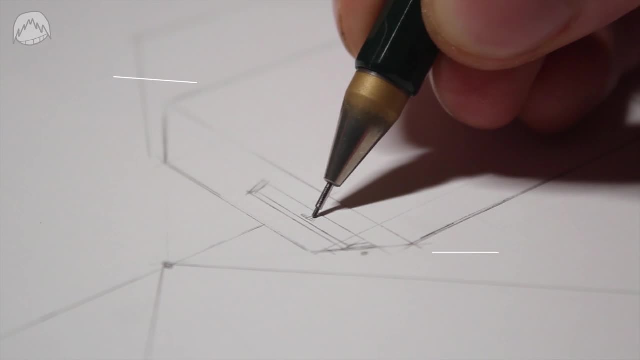 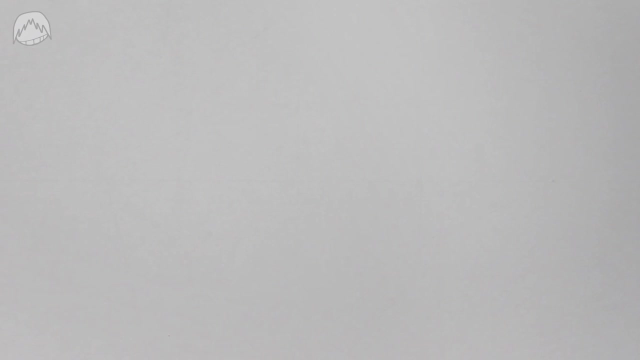 of our videos and like something new, please let me know in the comments. Good luck with the work. I hope to see you next time. Bye //. //. a second vanishing point to our horizontal line, And this means that the lines we drew horizontally. 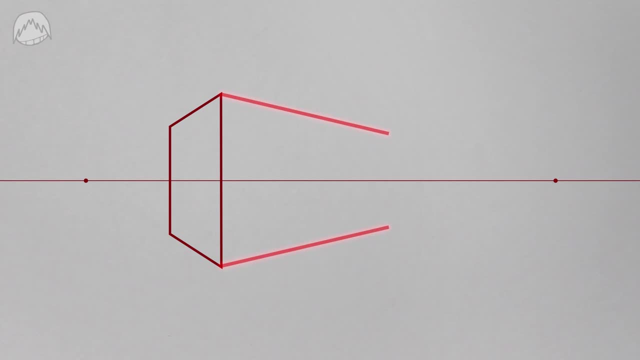 now points toward the second vanishing point. Now, I don't really know how difficult or complicated this looked, but let me assure you it's way easier than it looks Here. let's draw it together: You have your horizon line with two vanishing points. 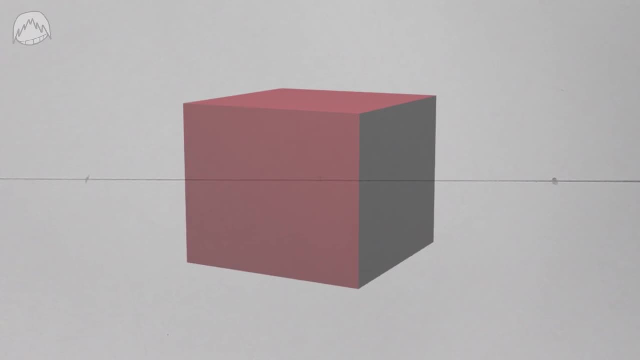 and we wanna draw a cube. that's about this size. You can now start wherever you want, but I always like to draw the vertical lines first. That way, I can measure how long each side is, in order to make my drawing symmetrical. 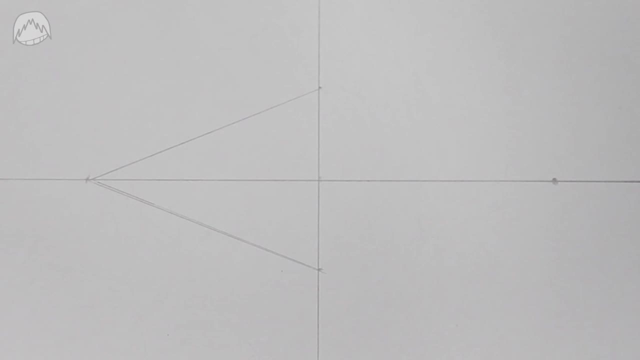 The lines on the left are now attracted by the left vanishing points and the lines to the right are now attracted by the right vanishing points And, just like before, you can cut the cube off wherever you want. but if it's supposed to be symmetrical, 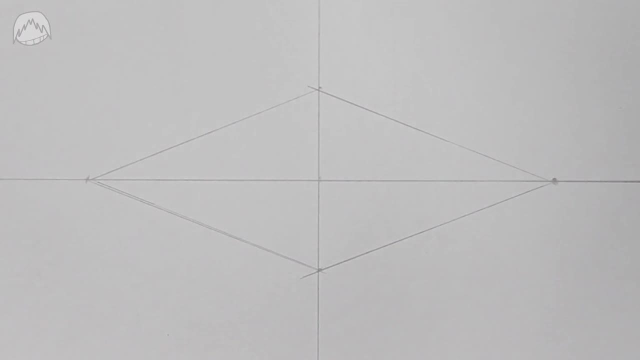 you need to measure it out first with your ruler, But don't forget to draw in the wireframe as well. Always remember that this can save you a ton of work later on. Like I promised, this was way faster than level one, wasn't it? 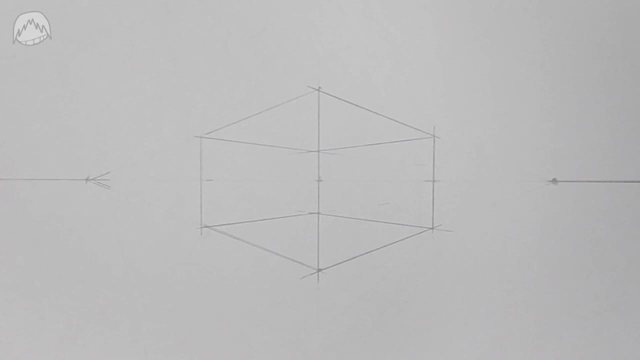 You can now go ahead and also transform this cube into a house by adding a street or, better yet, two streets. And how about the details? Well, let's have a look. We'll draw a door again, just like before. The vertical lines are simple, right. 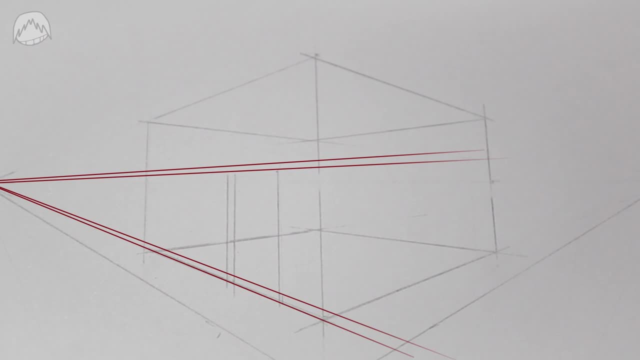 Then there's all lines that go towards our first vanishing point. So, just like with it before, And instead of just drawing horizontal lines, we draw those lines towards our second vanishing points. Now a personal tip from me to you. I like traditional pencils. 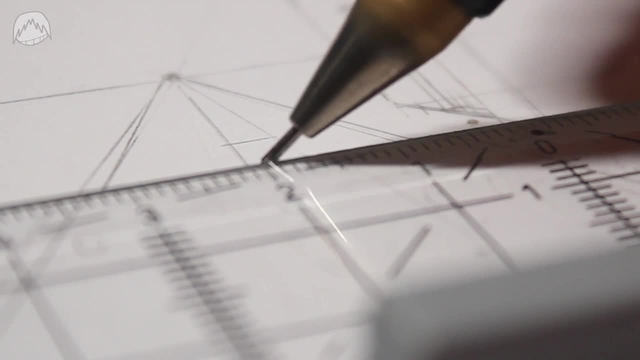 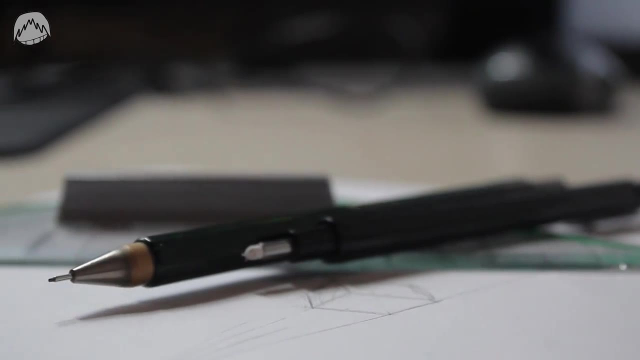 I really, really do And I like using them, but for drawings that are this tiny, I always prefer mechanical ones. They always have the same size and sharpness and are just more precise in general. If you wanna know where I got mine from. 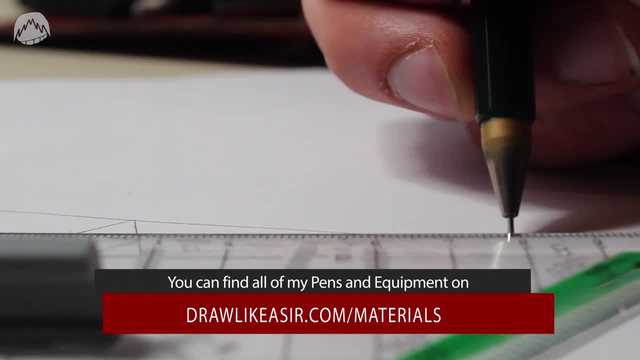 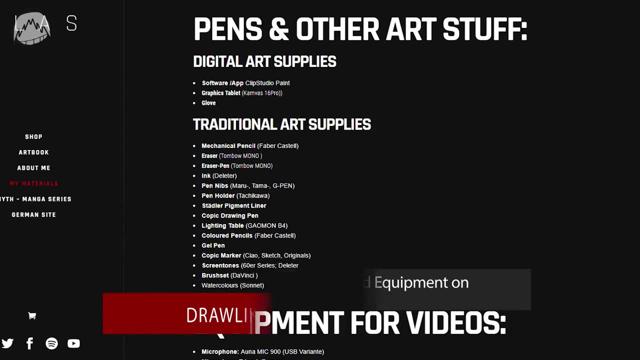 or what kind of ruler, eraser or other equipment I use. you can find everything over at my new website. There's a complete list of all of my materials I use for drawing and also for making videos. Also one last thing before we head to level three. 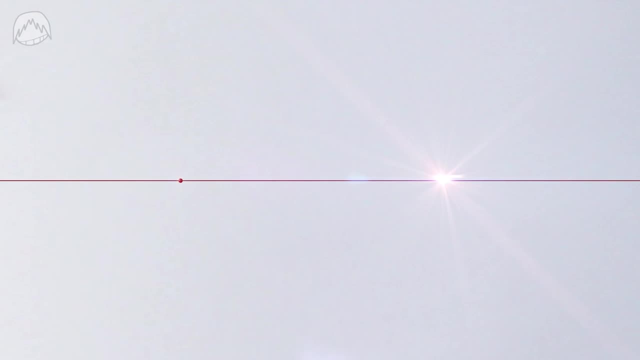 it's really important where on the horizon line you place your vanishing points. If they are too far apart, you might as well just use one vanishing point because it looks so flat, But if they are too close together it looks like your drawing is viewed. 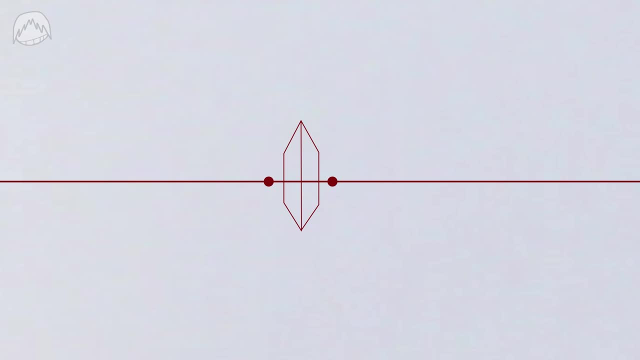 through the lens of a $5 GoPro, Except maybe you want that look, I don't know. By the way, I think the whole perspective thing with the horizon line becomes a lot more apparent here If the horizon line's at the bottom. 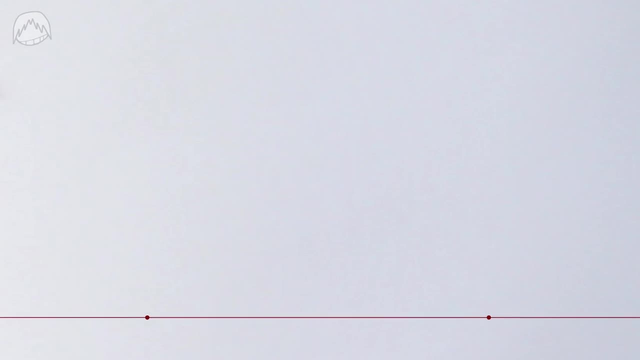 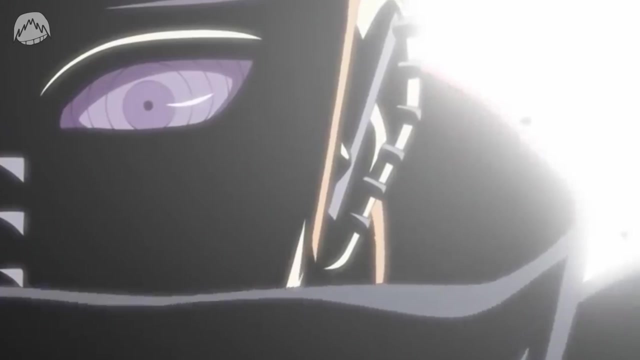 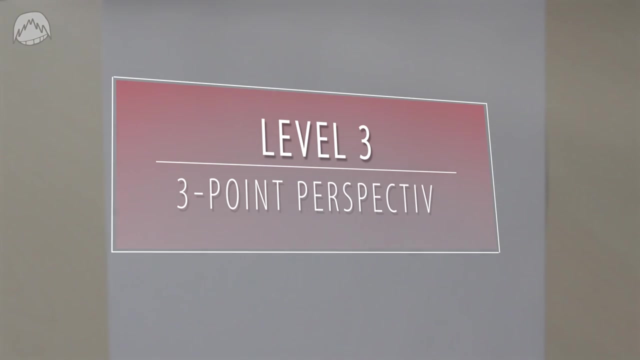 it looks like you're looking upwards, And if the horizon line's on top, then it looks like you're above the town and looking downwards like a bird or a plane or maybe Like you saw at the beginning. level three will be the shortest. 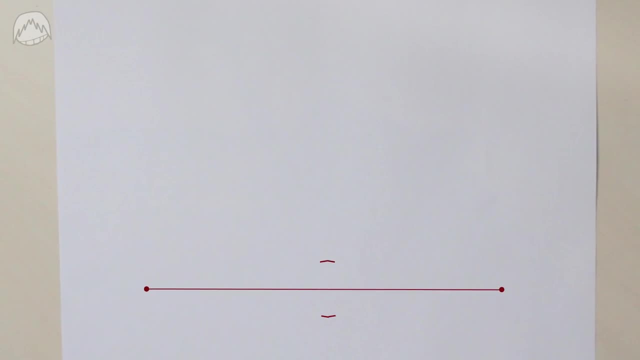 We already saw how the first two vanishing points are attracting the horizon lines like magnets. Before we just drew the vertical lines straight as an arrow. but now things will be a bit different, because now we have our third magnet, our third vanishing point. 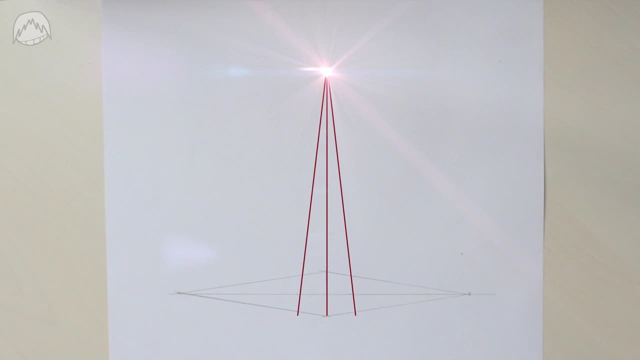 And this one doesn't even have to be on the horizon line, You can place it wherever you want. And this, my dear ladies and gentlemen, was it. You now know at least the basics of drawing vanishing points. There's still one thing left to do now. 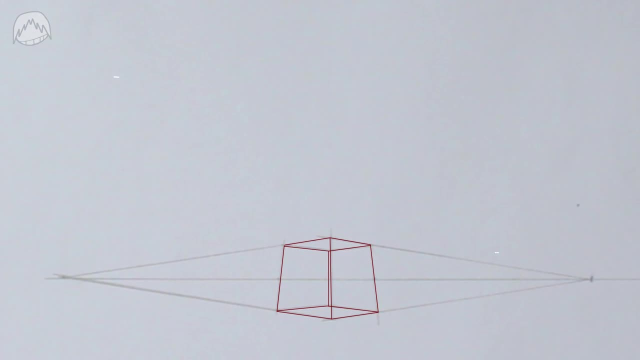 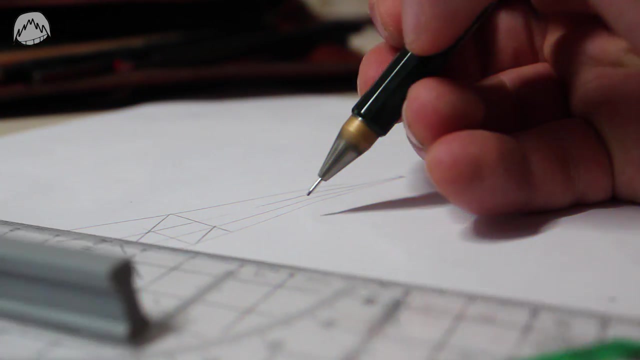 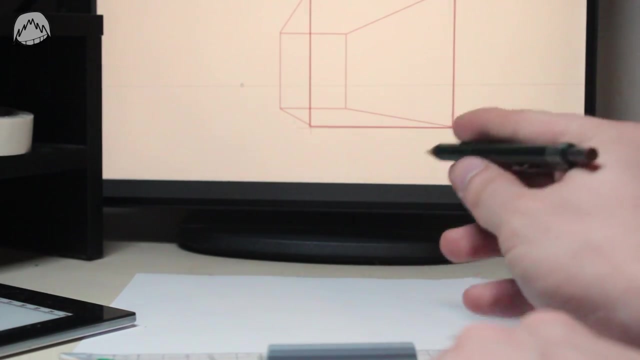 and it is to actually use this knowledge on your drawings, And I'll show you exactly how in the final level. So now I'm going to show you some things you need to know in order to use vanishing points in your art. But if there was something you didn't understand up until now, 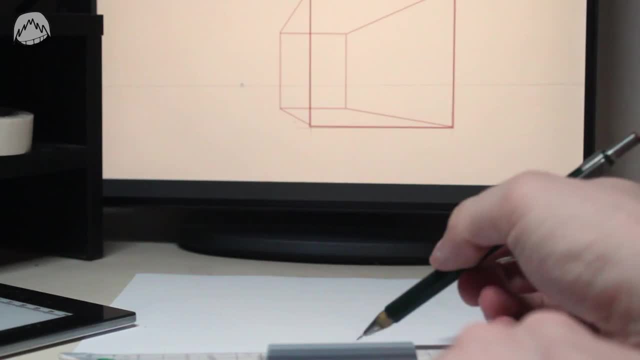 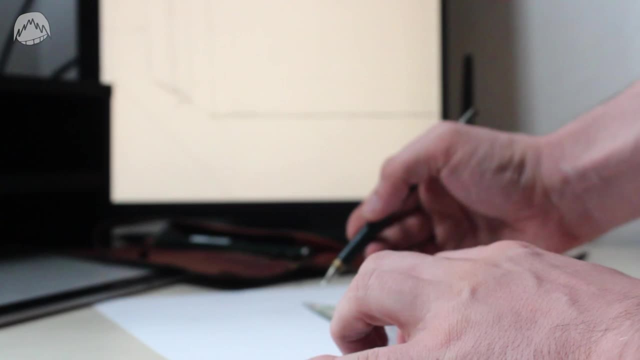 you should go and practice it first. I mean, that's what this video is here for. Just pause the video throughout and try to draw along with me, step by step. That way you can compare your drawings with mine to check if you did it correctly. 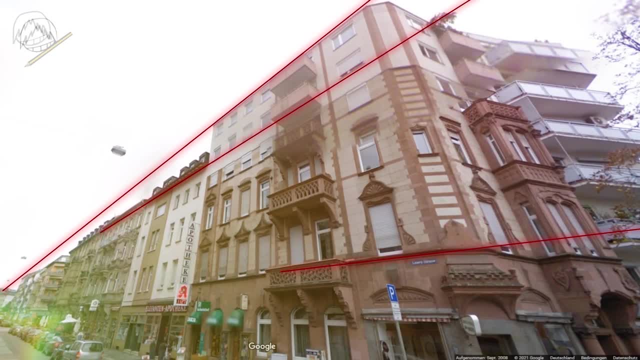 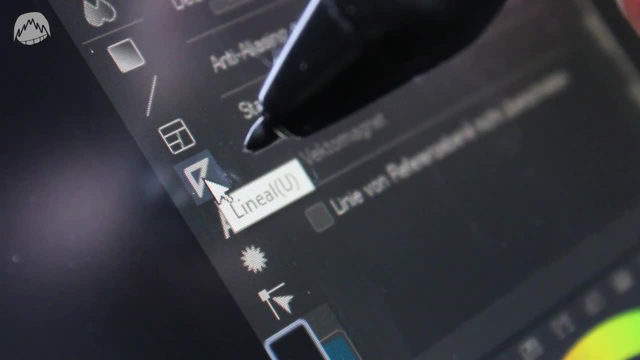 And that's too boring. You can also make a photo of your house or something and try to copy those vanishing points as a practice, And if you're drawing on your tablet, this might be even easier. Almost every software or app has a built-in ruler. 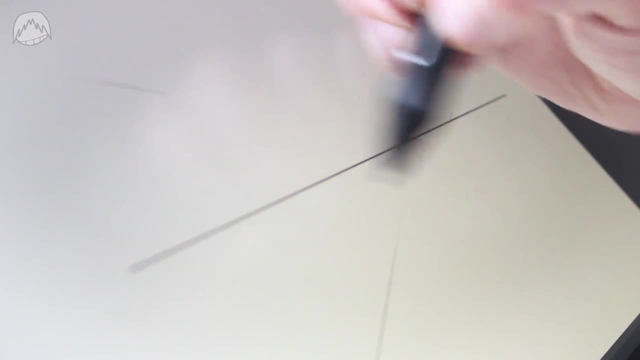 or something similar. And no, this isn't cheating or something. If you consider this kind of drawing assistance cheating, then let me know in the comments below And I'll see you in the next video. Bye, You should also consider a ruler cheating. 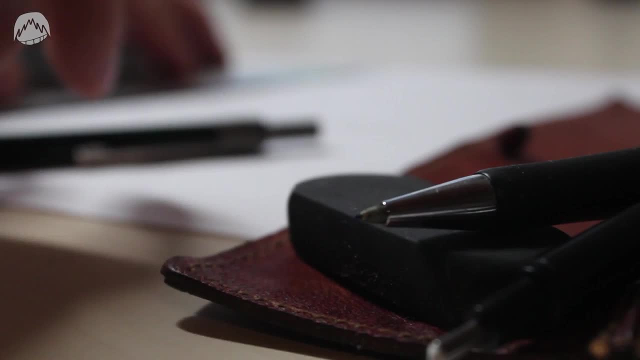 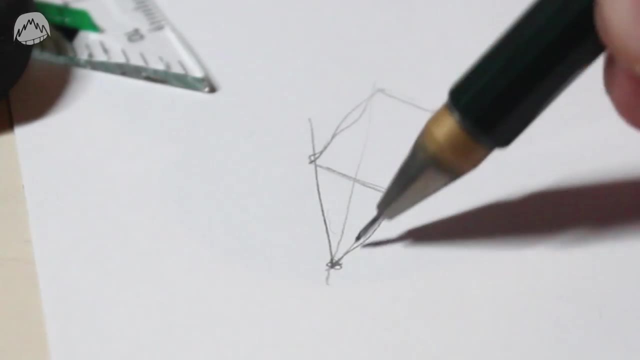 because it's basically the same thing when it comes down to it. And while we're on the topic of not using a ruler, maybe just try well, not using a ruler. I know how absurd this sounds, but that's how I do it. 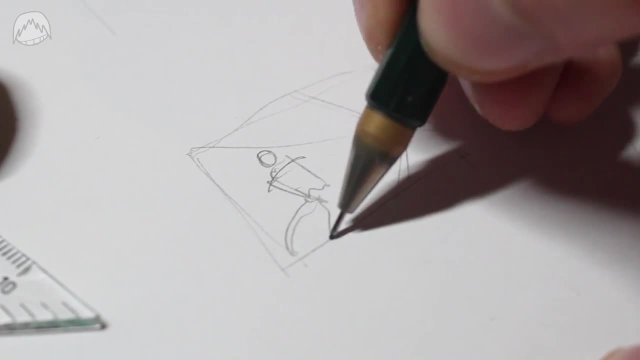 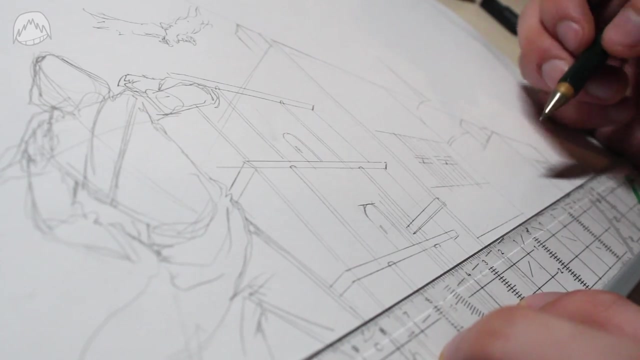 When I have an idea for an artwork, I always scribble down the rough sketch before using any rulers. Only when I draw the more detailed artwork comes the point where I use a ruler to check if everything's drawn correctly. Sadly, if you're drawing traditionally. 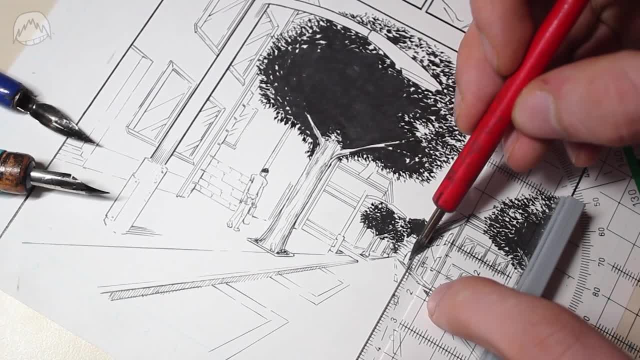 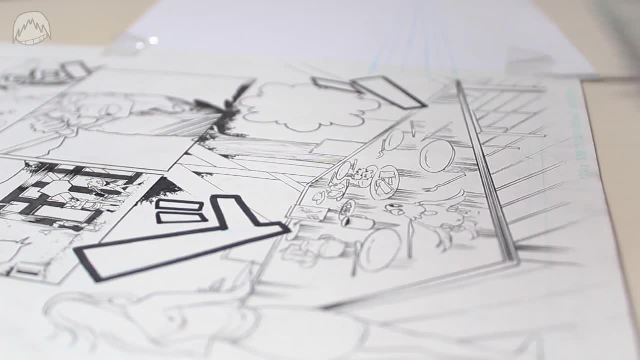 you'll have a lot more work with all of this. Let's see a quick example. Of course, I had to use vanishing points quite a bit over the last couple of years, for example every time when I drew furniture, But sometimes vanishing points are so far apart. 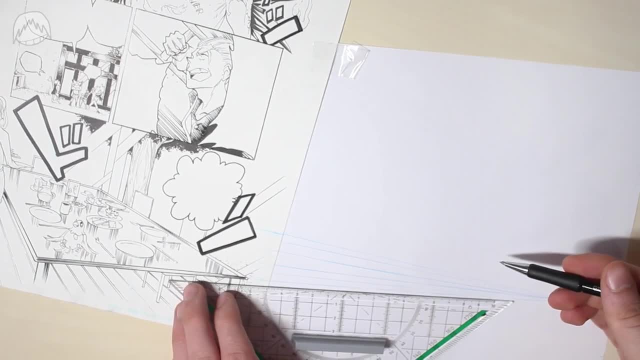 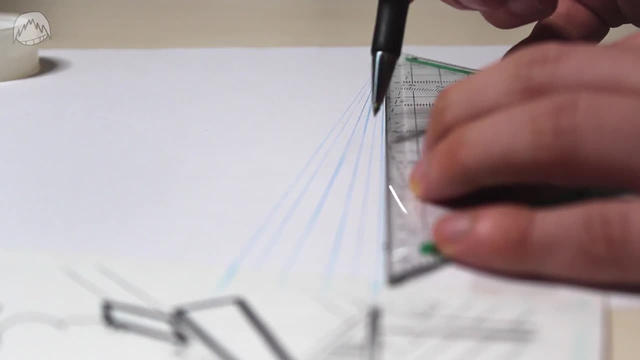 that you have to add another sheet of paper to even be able to see your vanishing points. And yeah, I'm afraid there's really no way around it. After a couple of pages I started fixating it. I'd advise you to do the same thing. 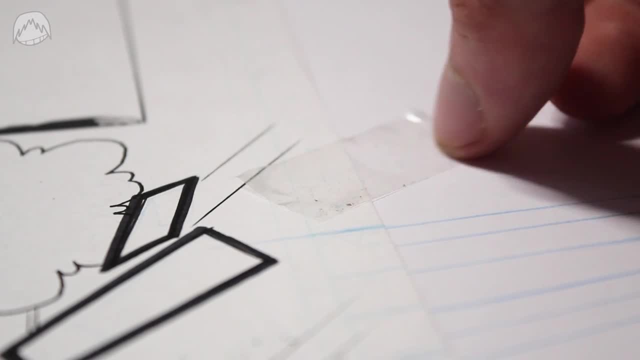 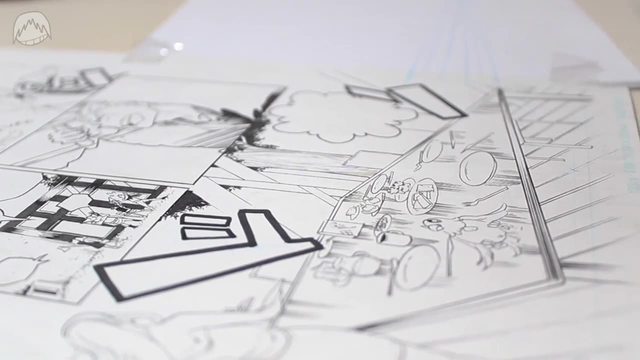 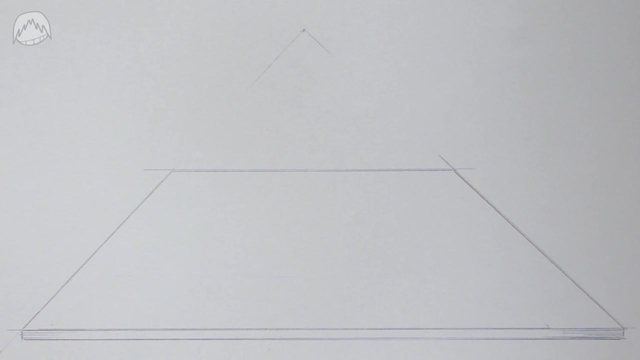 because, if not, your drawing will be utter chaos, Believe me. Oh, and if you've been wondering about how to draw objects that are round and not angular, well, just make them angular. I know this sounds like a bad joke, but it actually is not a joke, for a change. 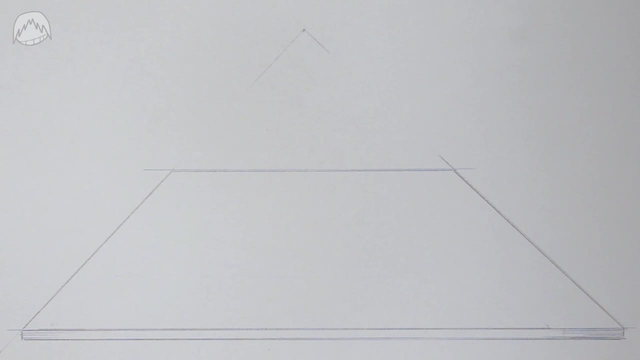 Let's also take a table, for example, just to make things easier with drawing a one-point perspective here. Let's say, we want to draw a simple plate here. Instead of just freestyling it, I draw a rectangle where I want my shape. 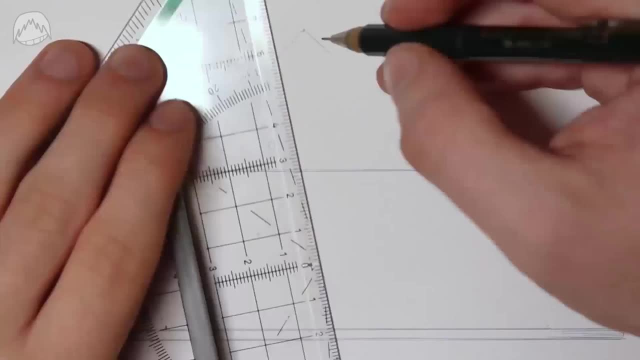 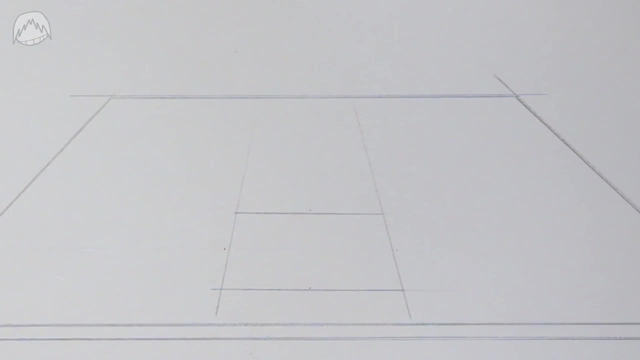 And right after that I mark the middle of each side, And now drawing a plate will be much easier than before, But of course it's still a pretty difficult thing overall if you're not very experienced in it. But this is at least how I would go about it. 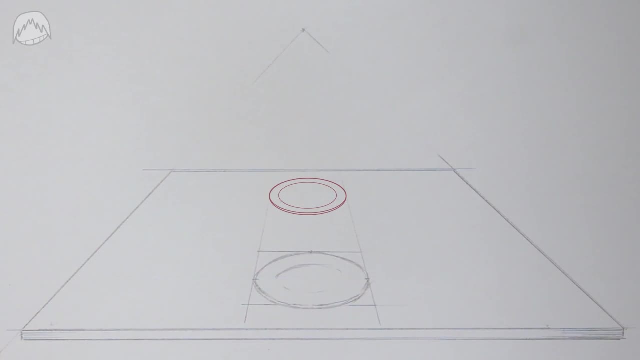 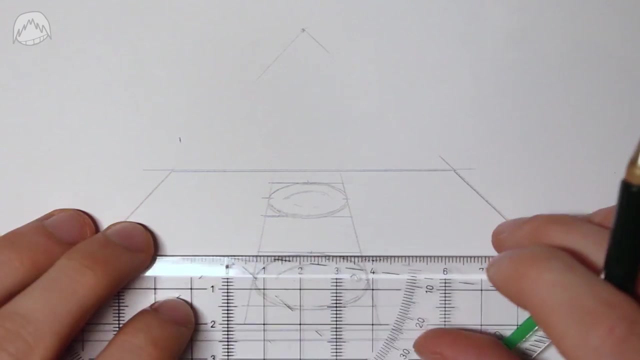 Also, don't erase the rectangle you just drew. You could use it as a guideline for, for example, a second plate, And if that wasn't challenging enough for you, you can draw more advanced forms, like, for example, a glass. 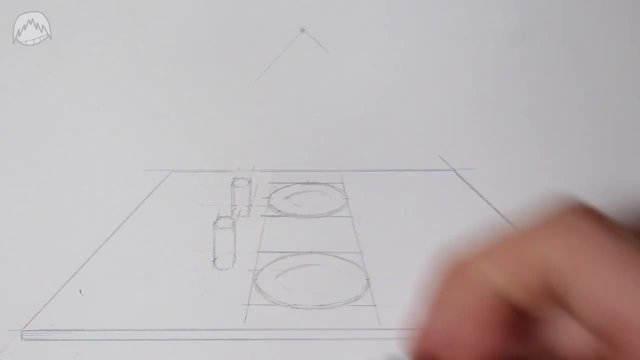 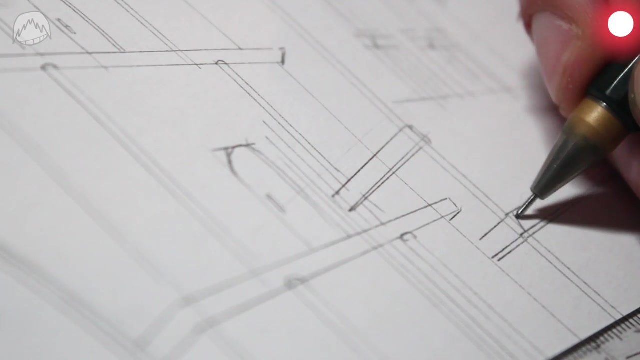 If you want to get into drawing more organic things in perspective, like humans, for example, I've already made a video about it And, with that being said, I have one last insider tip for you that will help you draw in perspective. So what's the secret weapon of mine? 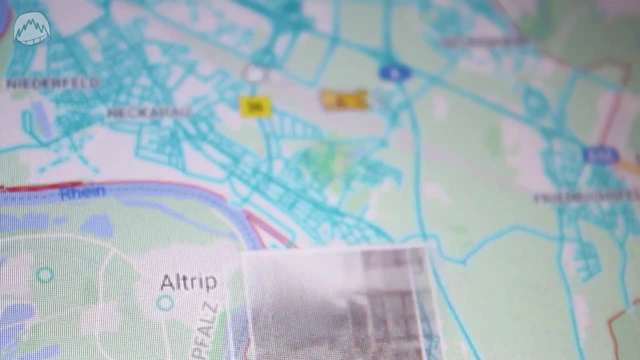 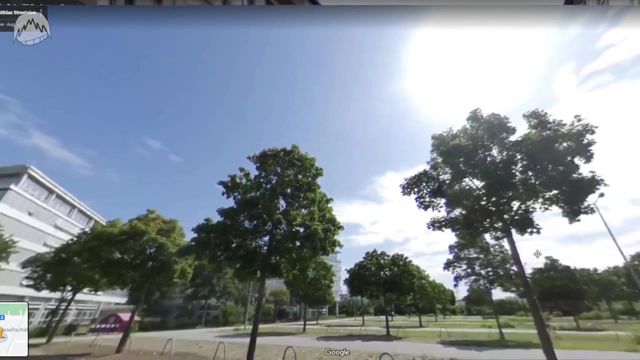 It's Google Street View. It's by far the best tool for practice in perspective and finding photo references. You can find everything here: Tall buildings, landscapes. you can find references for everything And you can even adjust the angle from where you look at it. 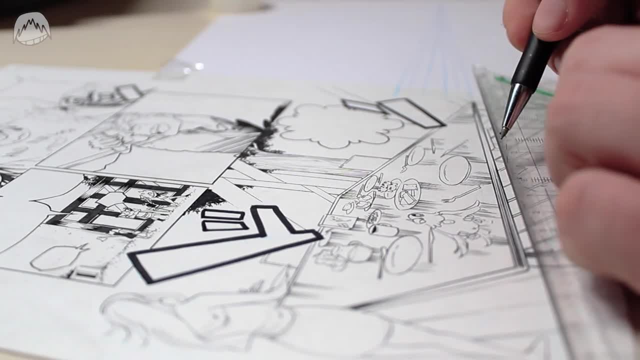 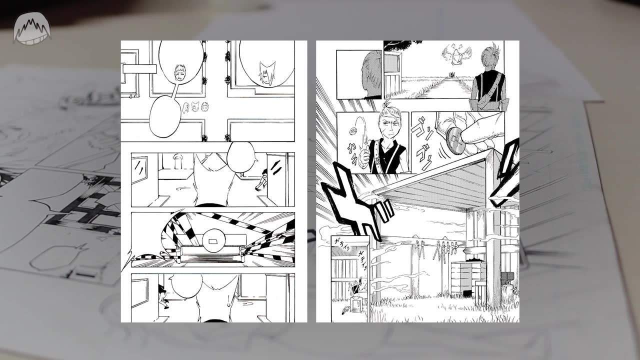 It's so damn good. If you don't believe me how good this is, here's a manga page I drew before and one I drew after. I practiced with Google Street View. Also, you guys keep asking about my manga series- Me and my story writer concluded it last year. 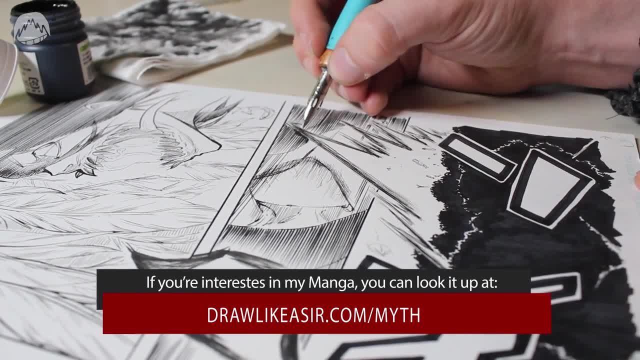 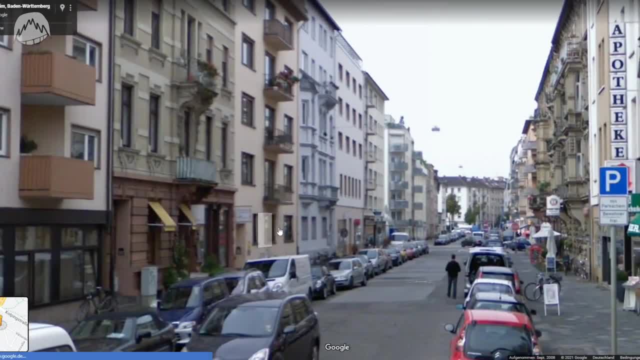 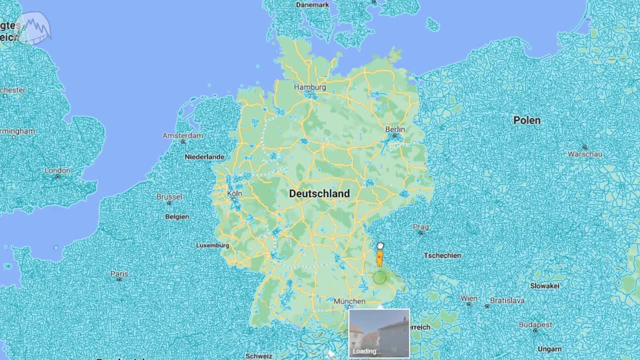 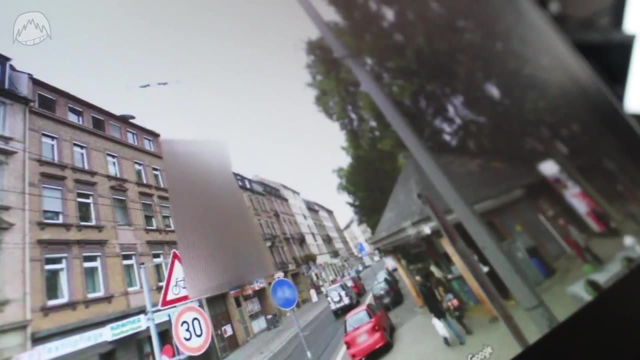 Anyway, about Google Street View. It's the best tool for drawing perspective that works absolutely everywhere. It's the best tool for drawing perspective that works almost everywhere. It's the best tool for drawing perspective that works almost everywhere. It's the best tool for drawing perspective that works almost everywhere.